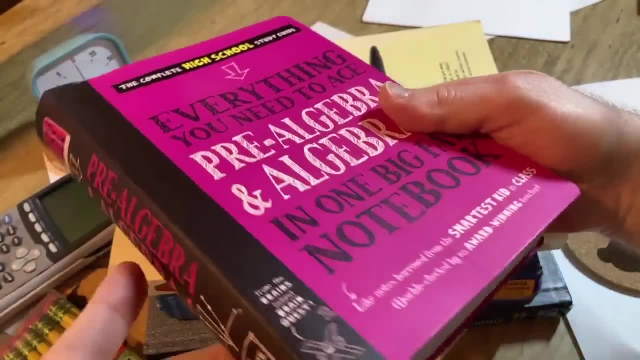 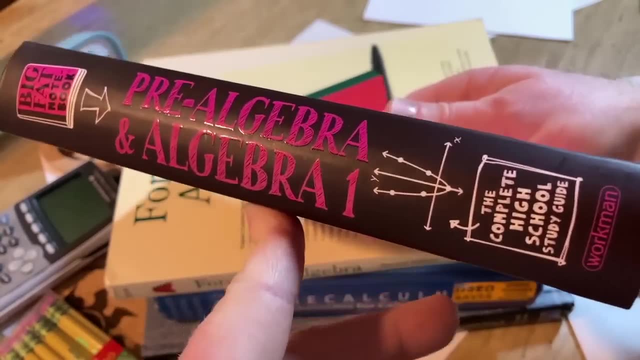 high school. Maybe you dropped out and you want to get started with algebra. This is a good choice for you. Or maybe you're in high school and you want a supplement. or maybe you're going to college and you just don't remember. But this book has everything you need from the very beginning. 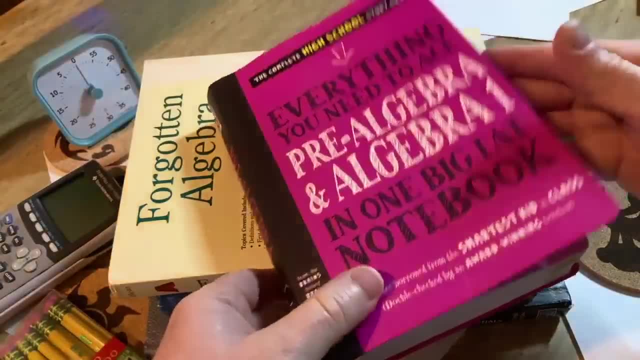 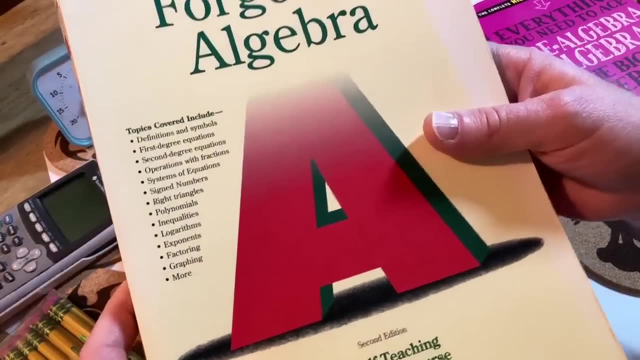 and it will help you learn basic algebra. Another really good choice which I believe is still widely available. This might be an older edition. I'm not sure This is Forgotten Algebra. It's got a really cool name: A self-teaching refresher course. Here it says this is a self-pacing. 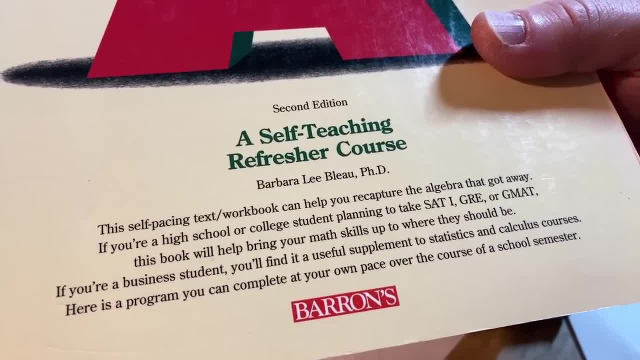 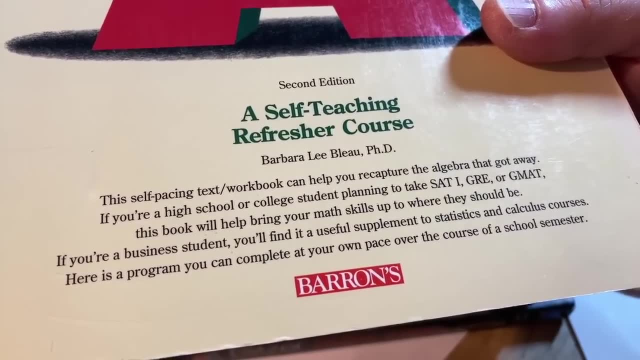 text workbook that can help you recapture the algebra that got away. If you're a high school or college student planning to take SAT1, GRE or GMAT, this book will help you bring your math skills up to where they should be. If you're a business student, you'll find it a useful supplement to 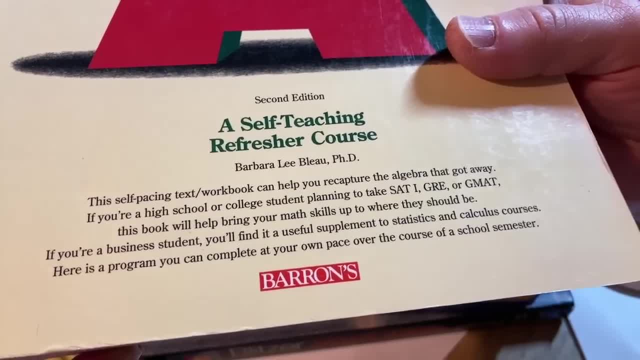 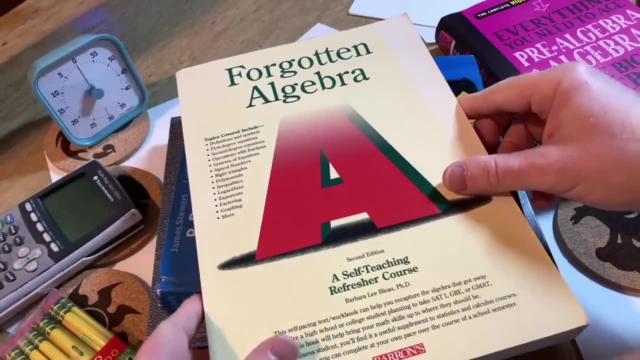 statistics and calculus courses. Here's a program you can complete at your own pace over the course of a school semester. I like that. they're being realistic. You're not going to be able to sit down in one night and work through this, unless, of course, you've had some math in the past. You would be surprised how. 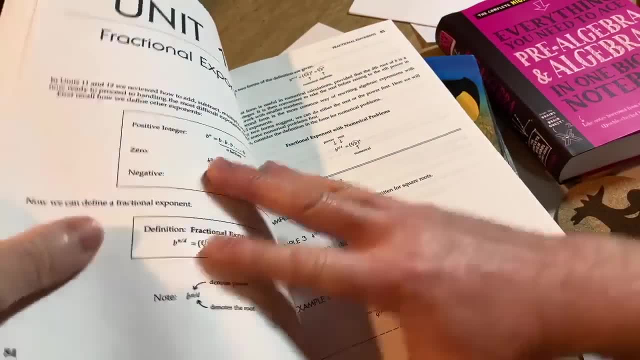 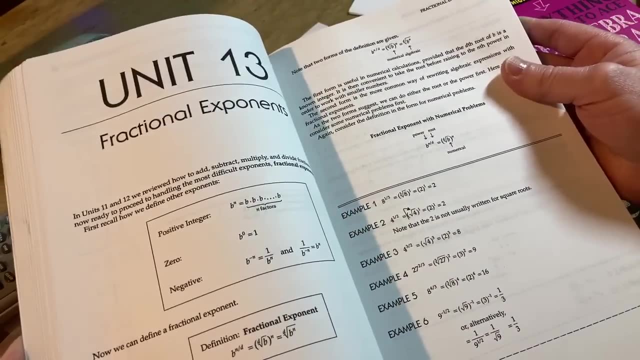 quickly the forgotten algebra returns to you. I always think that mathematics, learning mathematics, once you learn it and you forget it and you come back to it, it's kind of like muscle memory. You know if you work out in the gym and you stop working out. 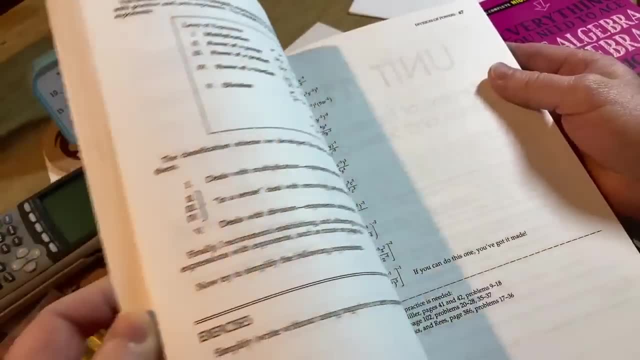 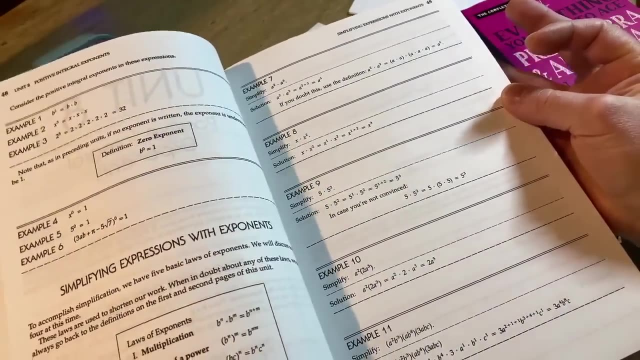 and then you start up again. your gains come quicker because you have that previous muscle memory, as they call it. So I think there's something similar with mathematics. You have that mathematics mind memory. Like if you've done math in the past, it seems easier to recall old. 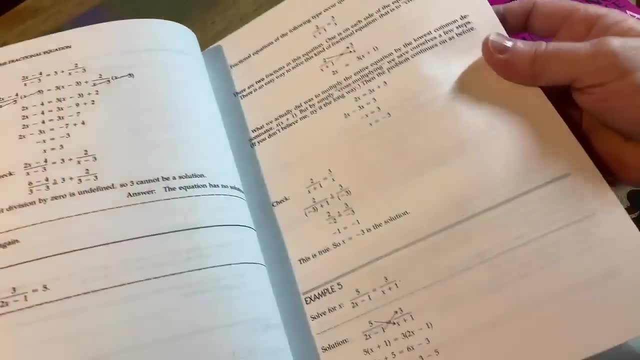 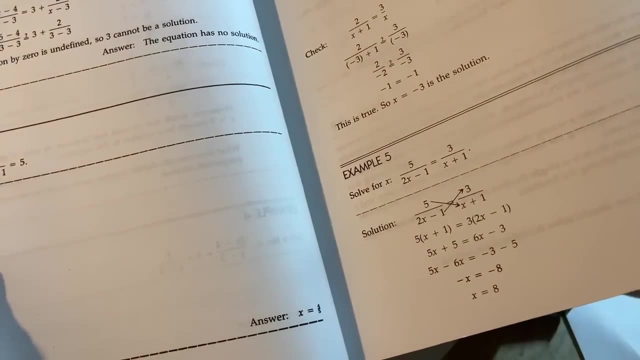 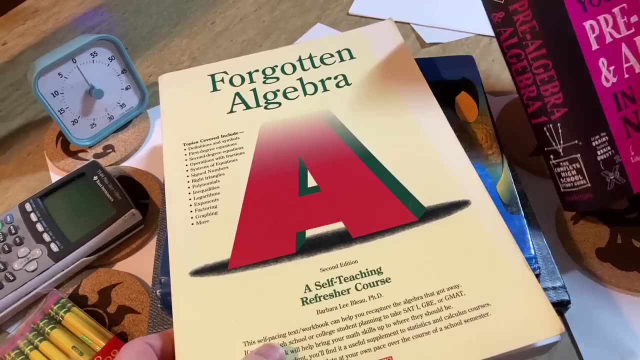 math than it does to learn new math. You can see, it has all the steps, It's got spaces where you can actually work through the problem and then it gives you the answer there, which is priceless. So a great workbook For someone getting started. So these two books, I think, are perfect. I'd recommend getting both. 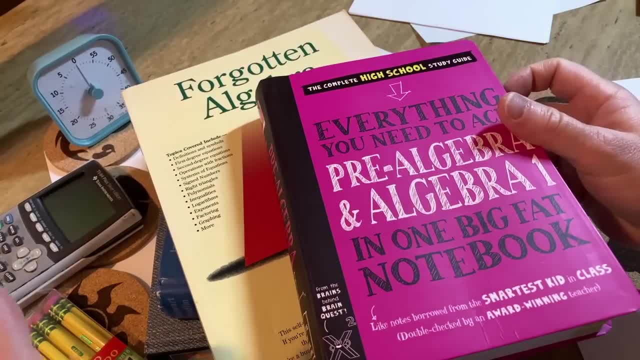 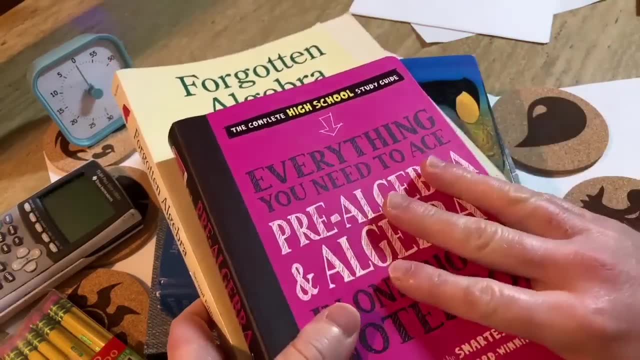 if you're trying to, you know, get started with basic algebra. By the way, I'll leave links to everything in the description in case you have trouble finding these online or something But worth buying. I bought them both. I bought this one new, So, yeah, very happy with it. 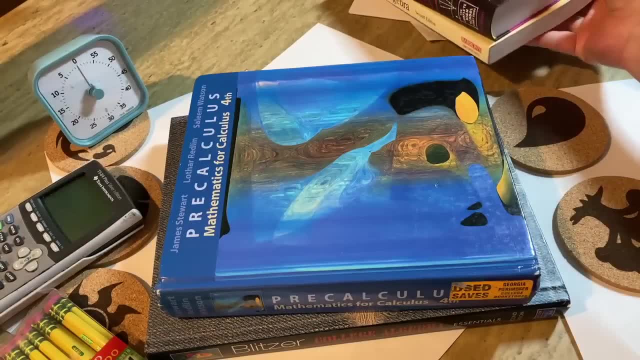 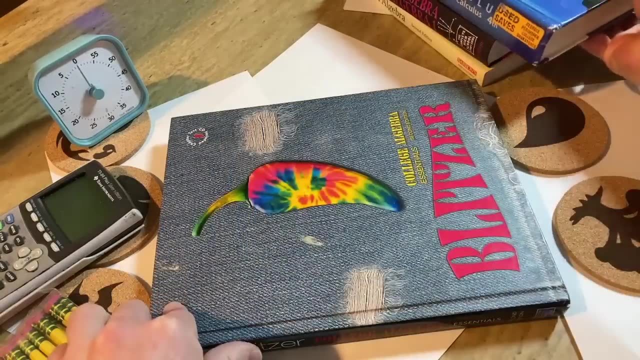 All right. So after you know some basic algebra- and so maybe you already know some basic algebra and you're thinking I already know basic algebra- I want something a little more advanced. So let's get to this book here. This is College Algebra by Blitzer, And this is the essentials. 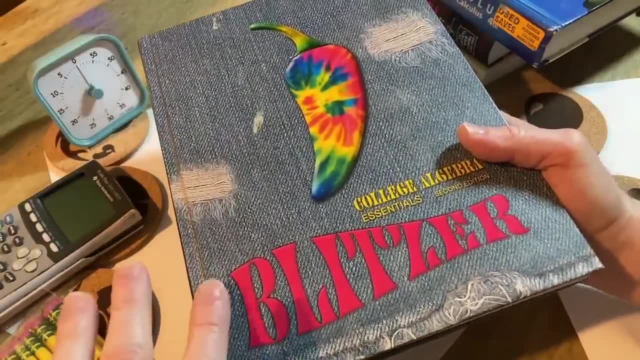 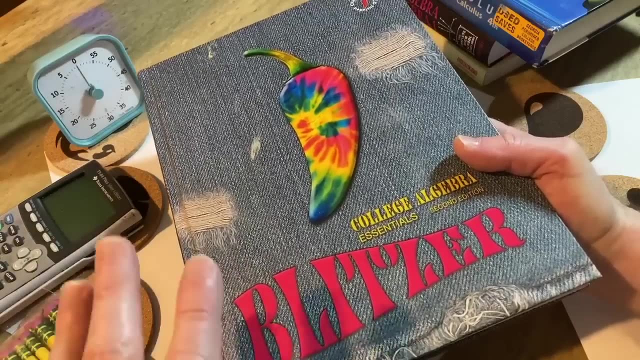 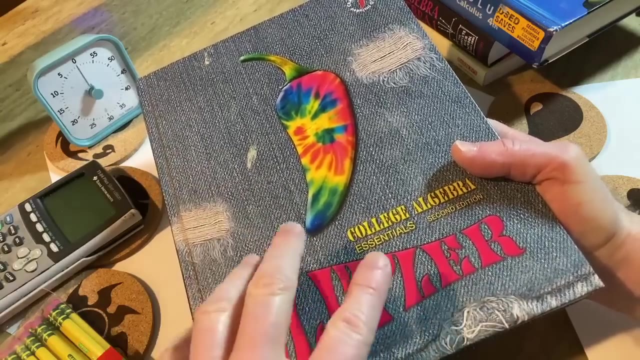 version. So this version has the essentials. So what does that mean? This version has what's typically taught in a college level college algebra course. I've taught college algebra. I taught it for so many years And we covered exactly what's in this version. If you have the 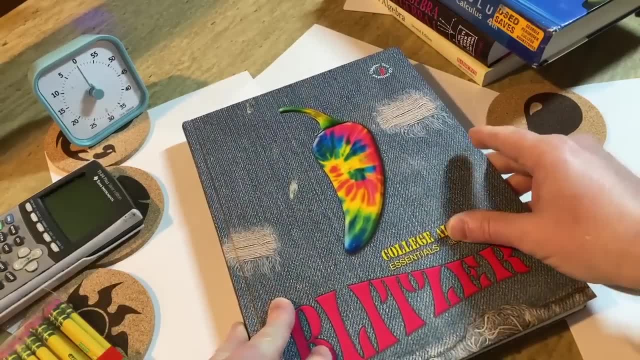 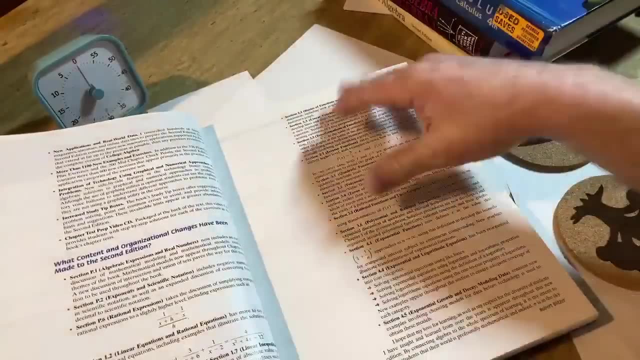 regular college algebra book by Blitzer. it has extra sections which I'll show you. I'll show you really quickly. So if you feel like you know some algebra, I say start here. I do think I'm not saying those other. 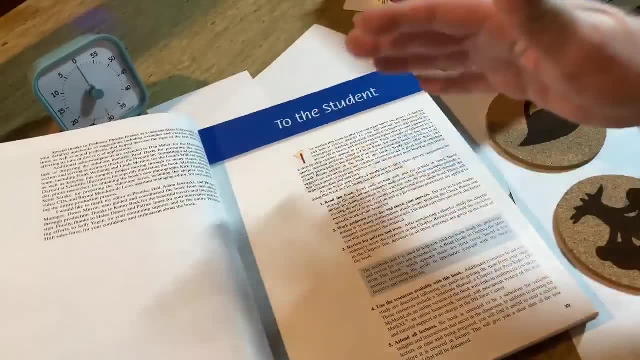 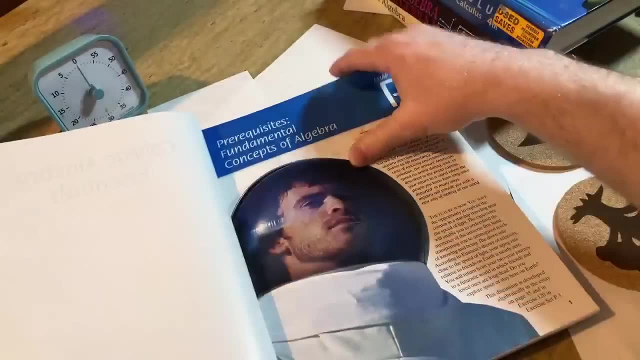 books I showed you were bad. but I think this is a better investment because this book has more math. This book has way more math than those other two books I showed you combined. It's just better, It's more advanced, It's college level mathematics. Let me just briefly find the 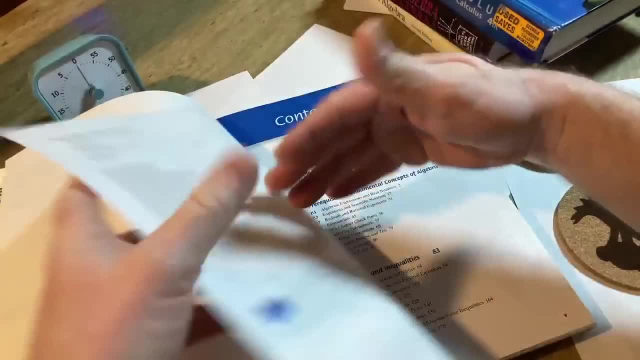 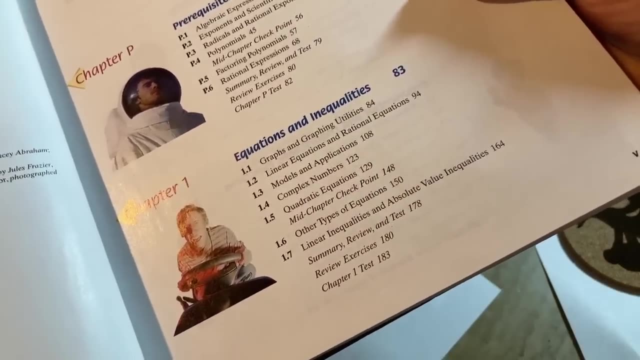 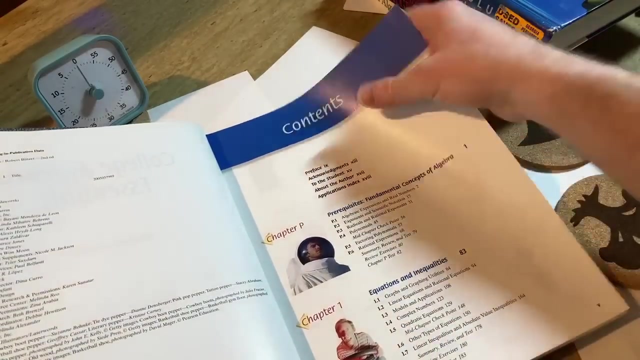 contents here so I can show you. I think I skipped over it. Here we go. So it starts with equations and inequalities. This is typically covered in a college level course. So if you go to college and you take college algebra, this is what you're going to cover. So this is typically the first test you 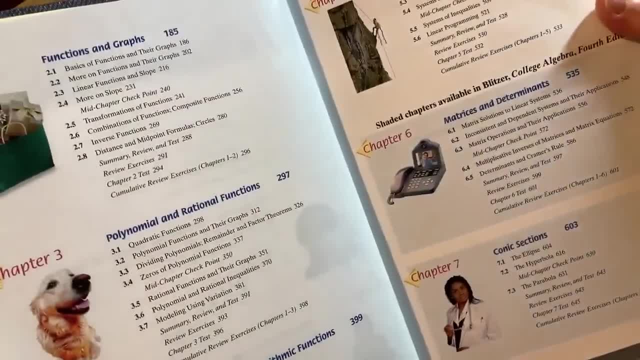 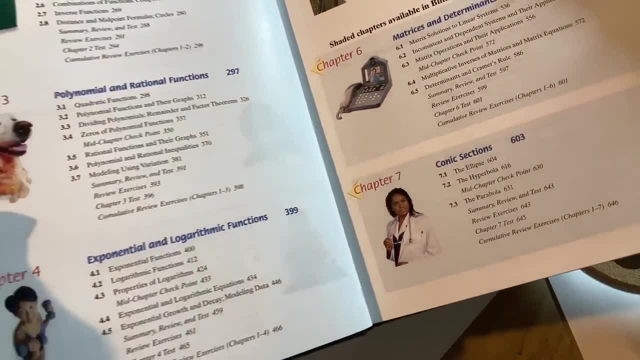 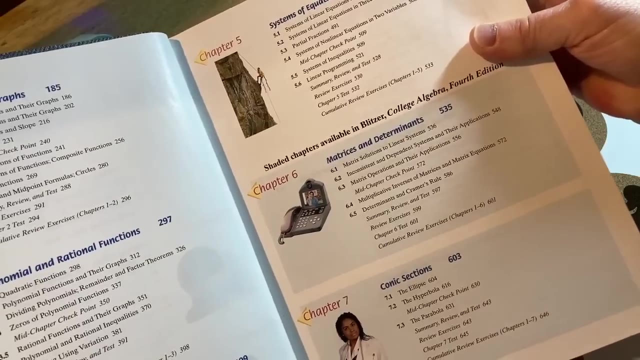 would take in college would be on chapter one, And typically the second test would be on chapter two, And then a third test, maybe chapter three, And the fourth test would be chapter four and chapter five together. So typically that's how it's done. So four tests, test one, chapter one. 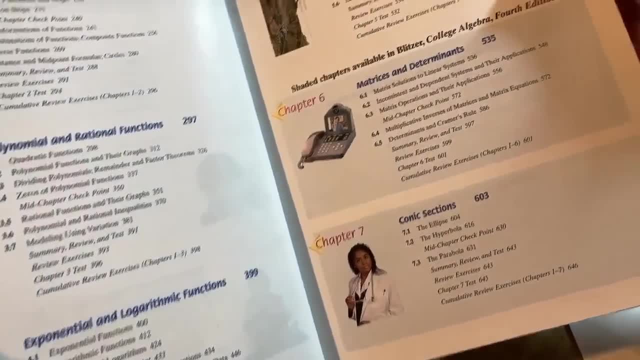 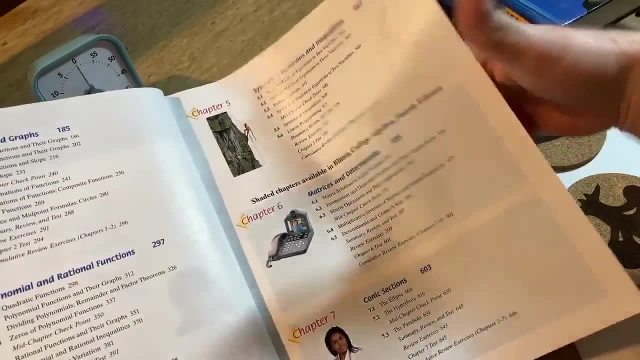 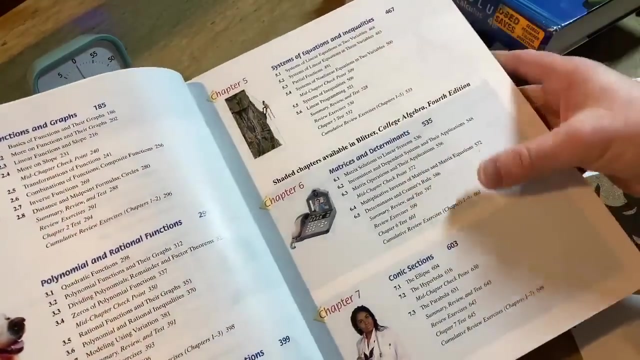 test two, chapter two, test three and then the fourth test, the last two chapters. Then you typically have a final exam, Whereas these sections here- matrices and determinants, conic sections- all of this stuff is typically taught in a pre-calc course. Now, when I took college algebra as a college student, I actually covered. 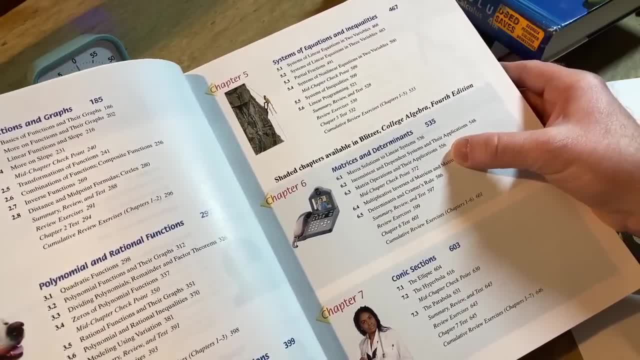 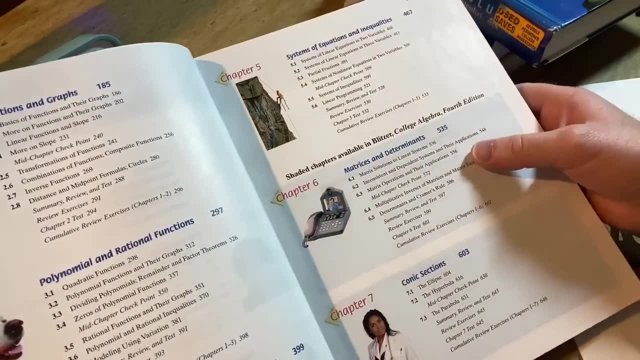 matrices and determinants, which was kind of interesting. My teacher decided to cover that, So it's optional. Note that these are available in the regular version. So you might be wondering why didn't I show you the regular version? I own the. 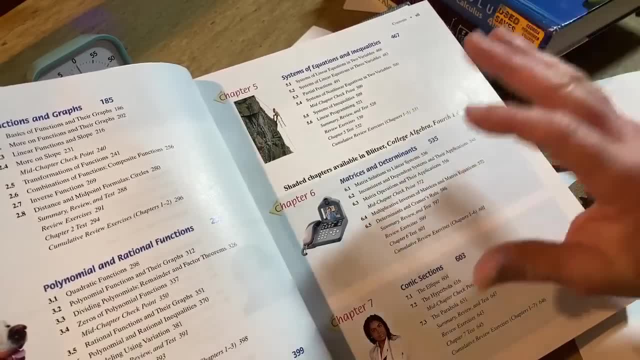 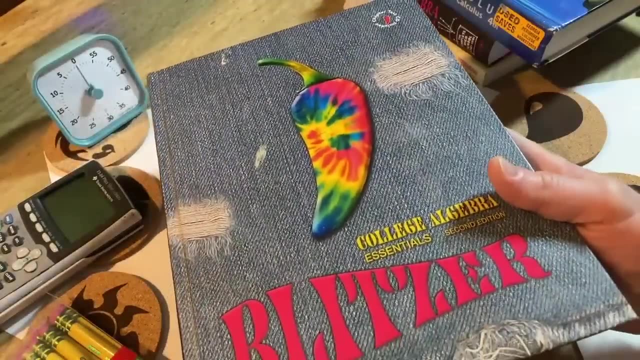 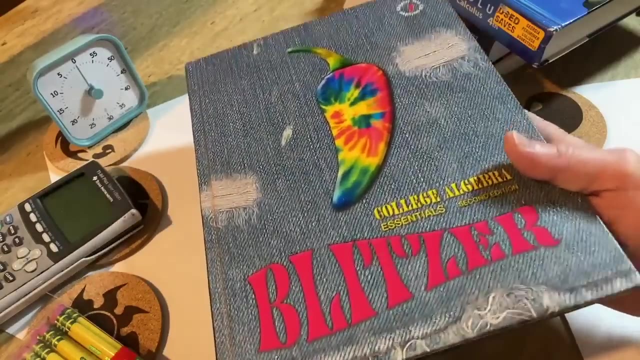 regular version of this book. I actually own the instructor's edition, But the regular version is more expensive, Like brand new, this book- and I'm pretty sure there's a newer edition, this is an old edition- is less expensive. So if you get the essentials version you can save money, But then you're missing those topics. So that leads me to the. 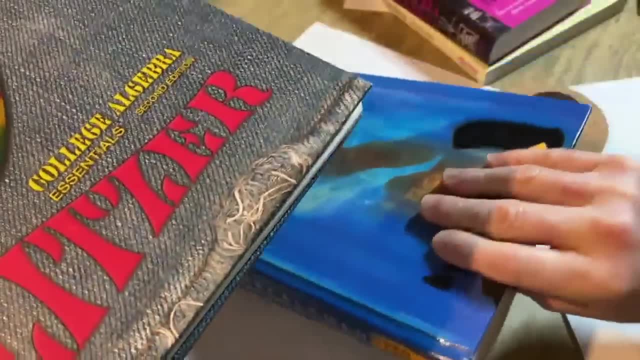 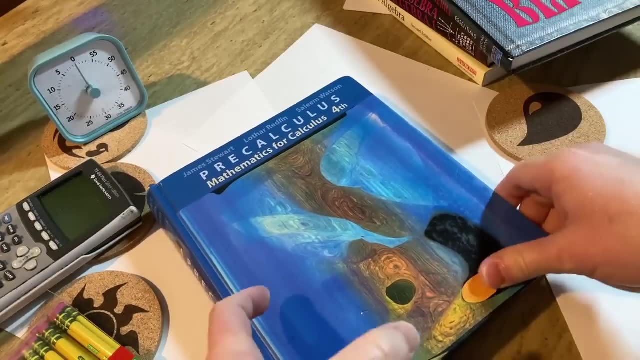 next book, So maybe you already feel like you know plenty of algebra. Here we have what's called a pre-calculus book. I used to have this friend on the internet. We used to chat all the time in a math chat room in the early 2000s. 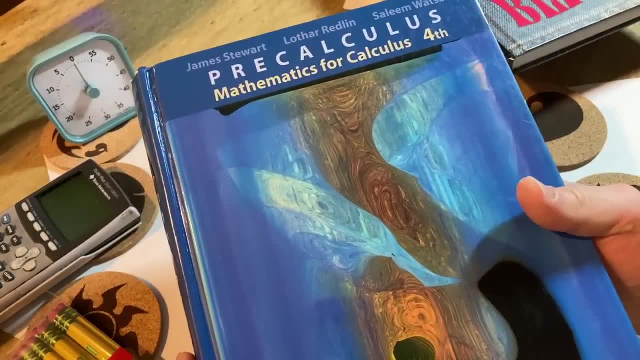 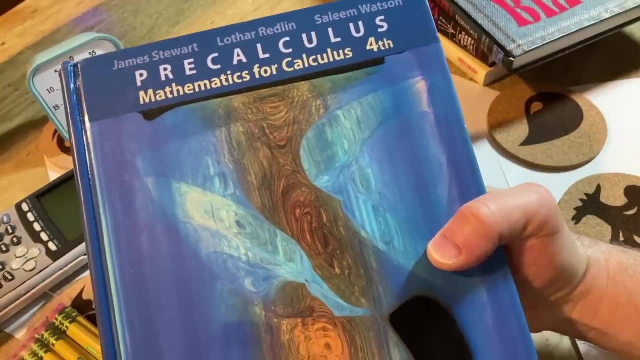 He was a really cool guy. He was a math major from the University of Waterloo And he was a genius And he always had a problem with the name pre-calculus. He would say: what in the heck is pre-calculus? Why do they even call it that? 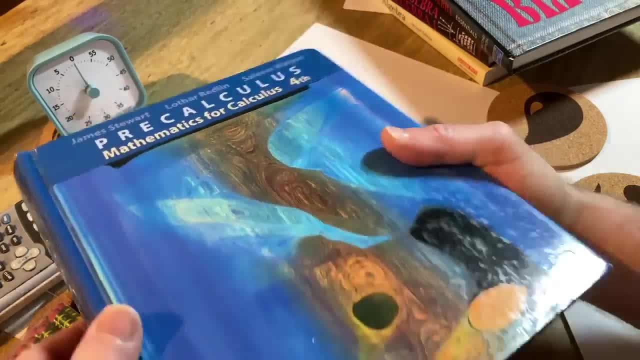 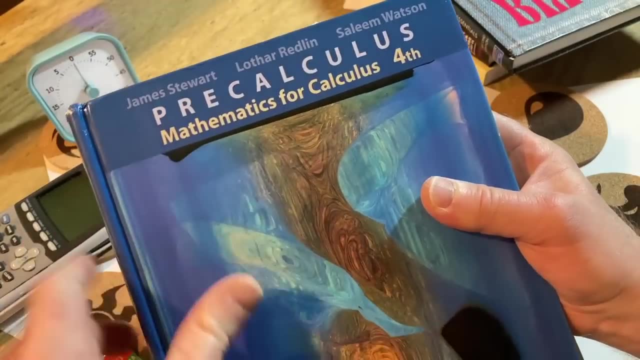 You know it's basically algebra and trigonometry. So a lot of books titled pre-calculus, basically, are titled algebra and trigonometry. This one's written by James Stewart rather than Watson. James Stewart was a very famous mathematician. He was a 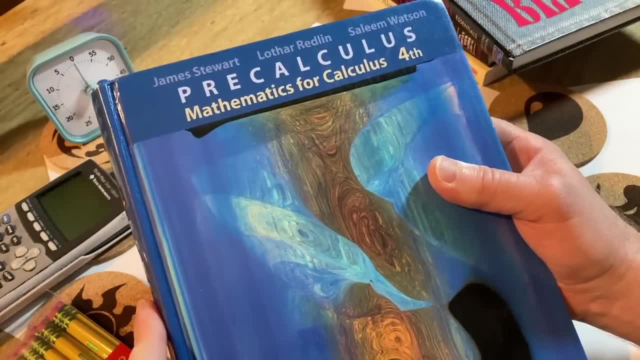 Canadian mathematician. He passed away several years ago. He was a very famous mathematician. He was a very famous mathematician. He was a millionaire from — he became a millionaire from writing his famous books, In particular his book Calculus is. 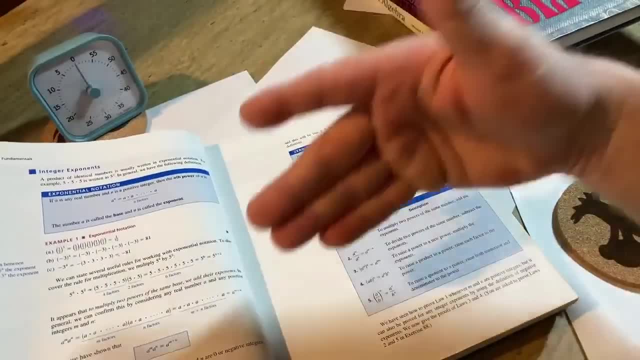 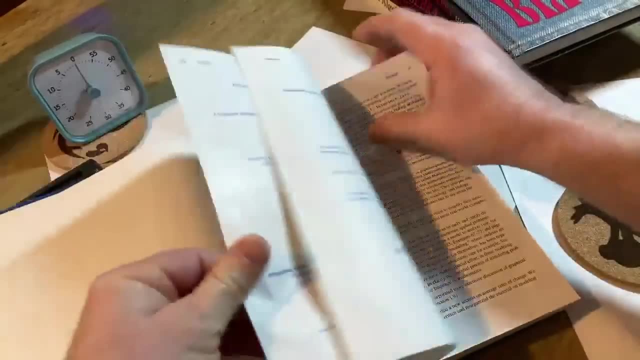 super famous. It's an awesome book And it's still used today. And this book is still used today in colleges, So this book would be used to teach like a pre-cal course or a trig course. Again, a worthy investment in my mind, this book, because of the knowledge it contains. 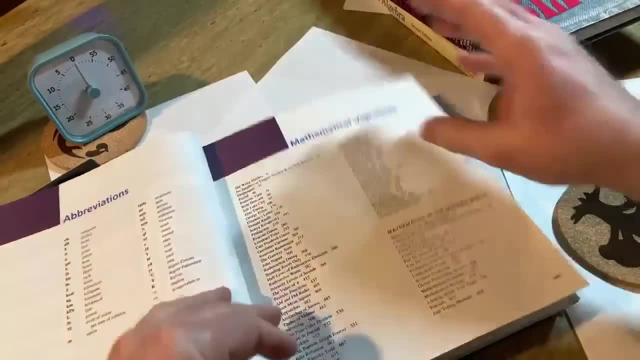 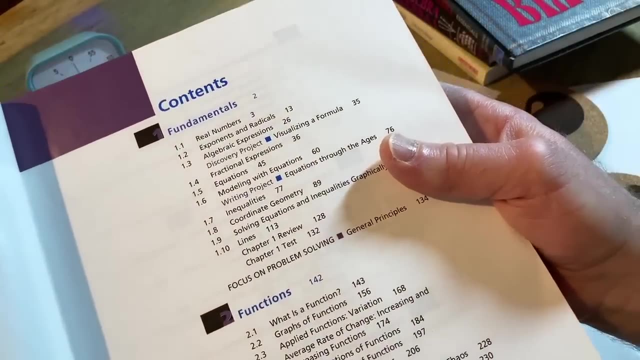 And it has a lot of the same topics that you saw in the other books, But it's a little more interesting. And it's a little more interesting because it's a particular book that I'm going to be highlighting: death, like some of the exercises are harder, some of the examples are harder. so, fundamentals. 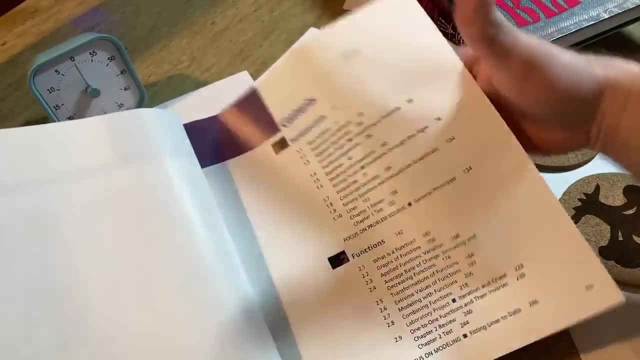 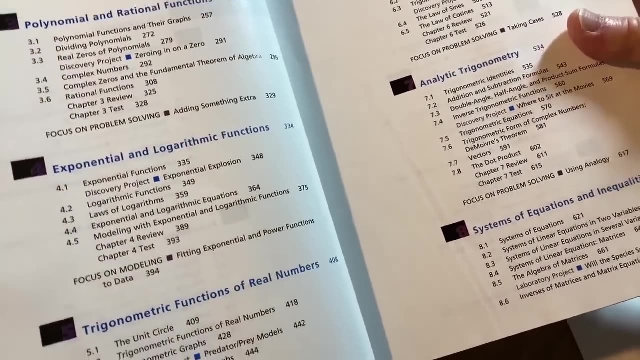 functions. they're very similar to the college algebra book: polynomial and rational functions, exponential and logarithmic functions, so stuff we saw earlier in the college algebra book by blitzer. and you've got trig functions, so it's got trigonometry as well. so this will prepare. 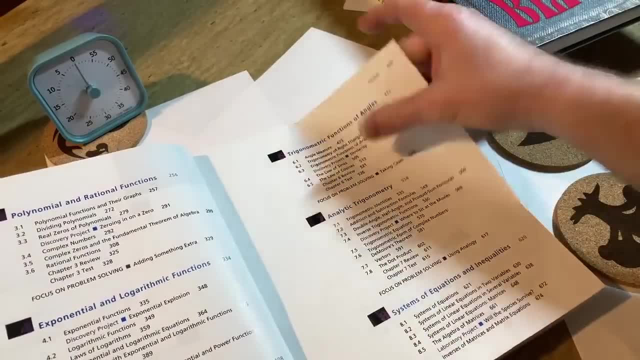 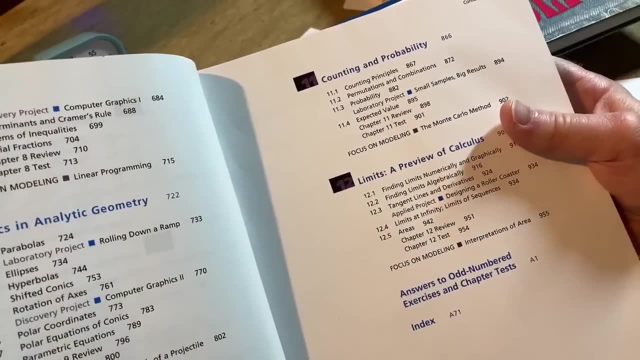 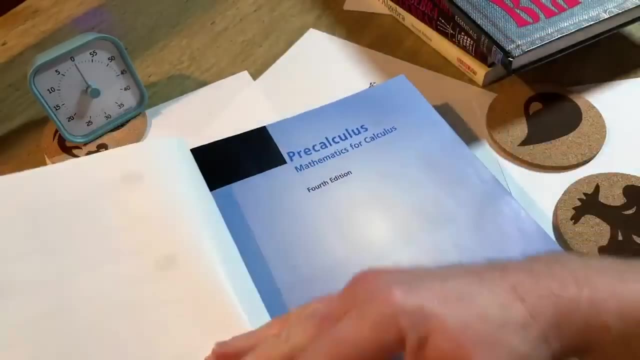 you for calculus, and then systems of equations and inequalities, some geometry, so these are conic sections, sequences and series, and then counting and probability. so very, very similar to the blitzer book. by the way, these books all have answers, at least to the odd number problems, so they make a great choice for self-study. so in my view, this book here, this pre-calc, 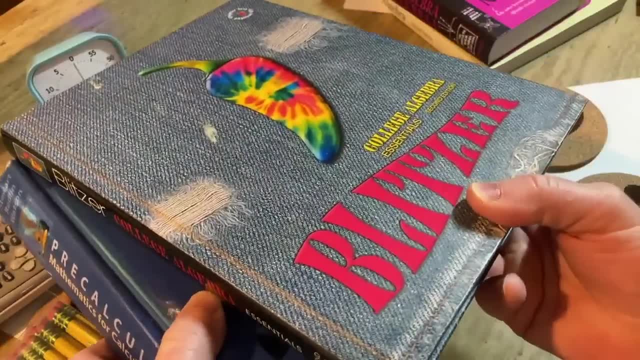 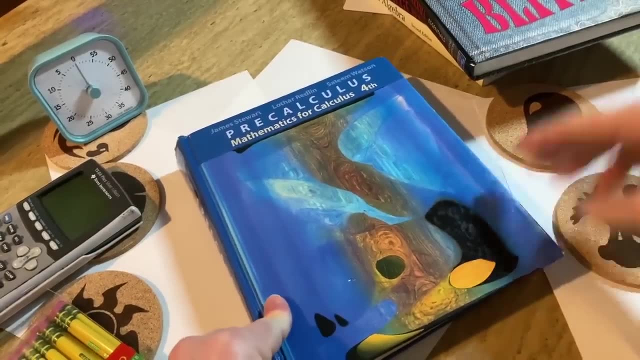 book and the college algebra book by blitzer are a better purchase than the other two books i showed you at the beginning. but if you need to start from the beginning, you definitely want to get you know one of those first two books i recommended, which were um this one here: so if you're interested in that, you can go to the link in the description box below. and you'll find a link to the book in the description box below. so if you're interested in that, you can go to the link in the description box below. so if you're interested in that, you can go to the link in the description box below. 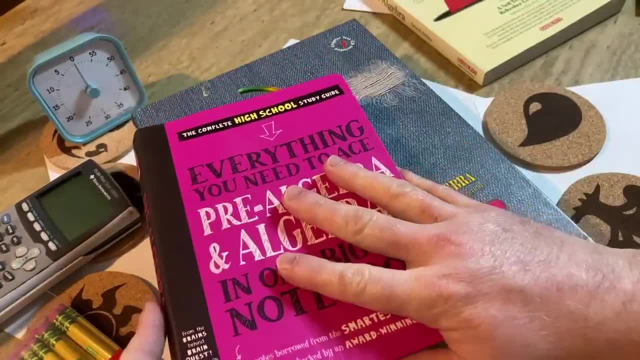 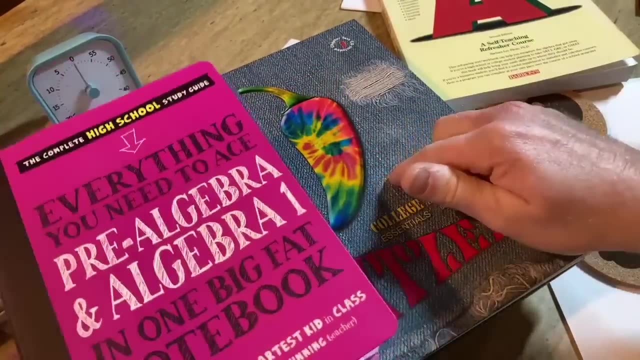 your math is really weak, you know. if it's really bad, get this, okay. uh, don't, don't just jump into the college algebra books. typically students who take uh courses in college- algebra in college- they struggle a lot. um, when i took it, i struggled a lot. i ended up getting, i think, a- b in the class. 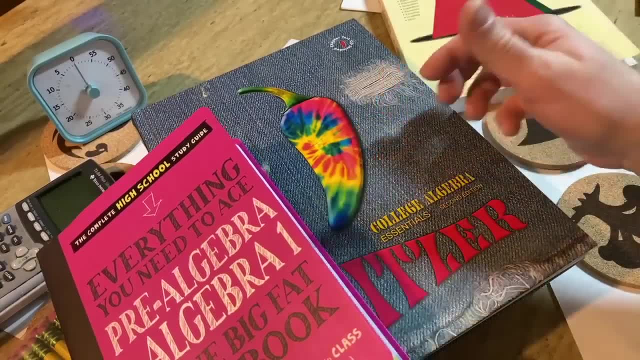 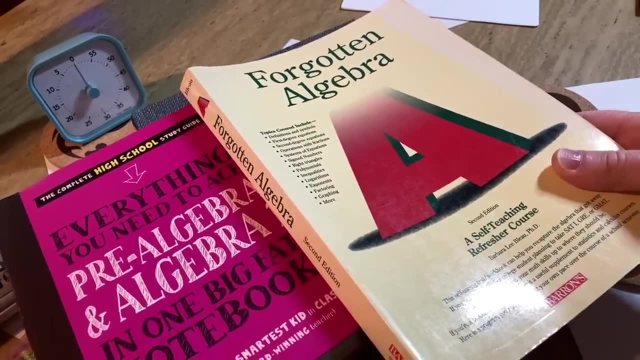 and it was just so difficult for me to learn logarithms. i struggled, i just had a really hard time. so maybe start with one of these two, if you know, if your math is really rusty and it's been like a long time since you've had math, so after you get through all, 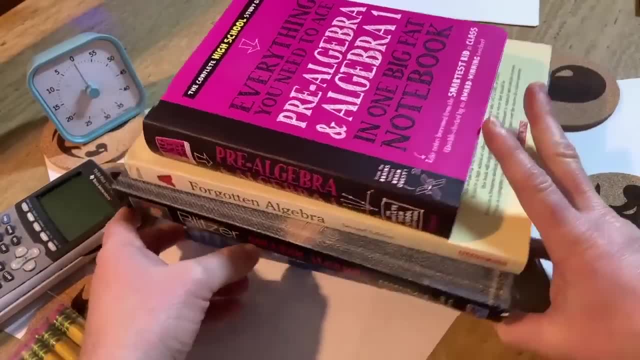 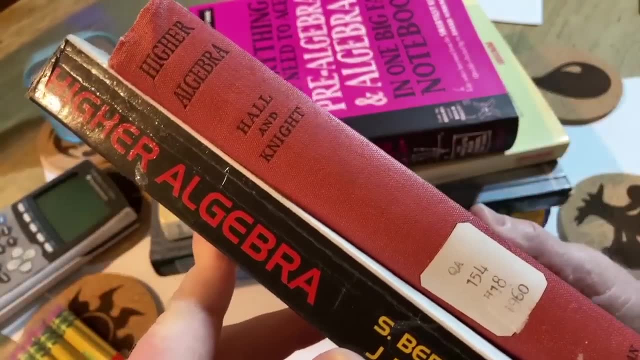 of these books. it's time to really get into some fun. and here we have two other books which are not used in the united states of america today. they're both called higher algebra. these books are used in india. i'm pretty sure these are used in india because, uh, these books, uh, were referenced. 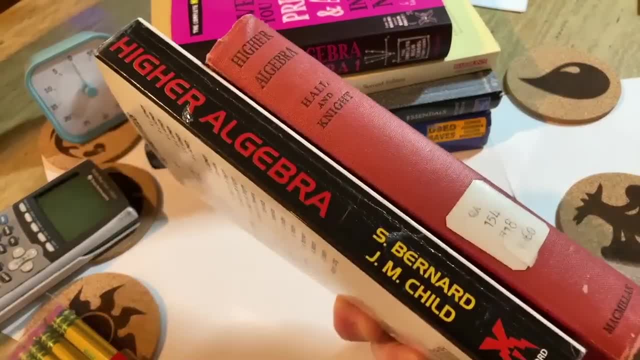 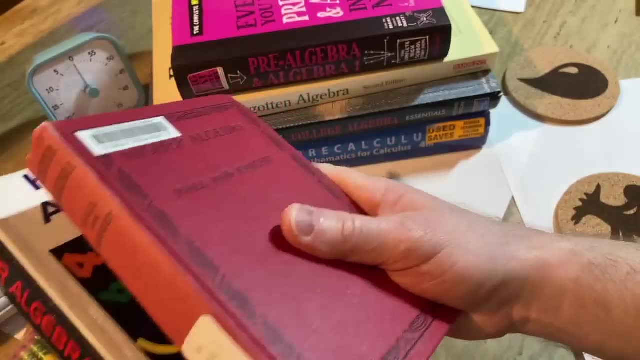 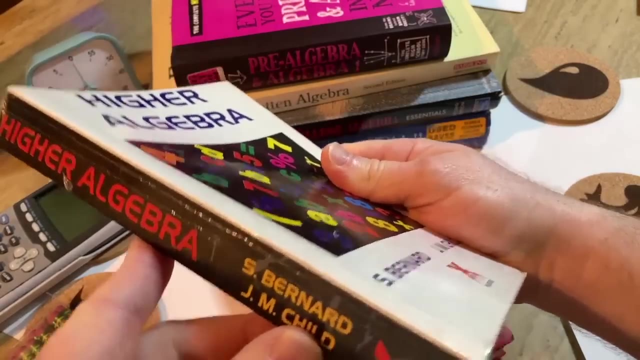 multiple times on my other youtube channel, the math sorcerer, people would leave comments, uh, and ask me about these books- people from india, and apparently these books are used there and i think that's amazing because these books are super hardcore. so this is an old book. uh, this book actually came from india. i bought this from india. it was 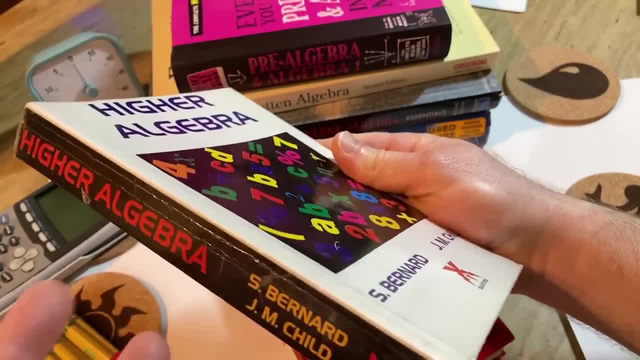 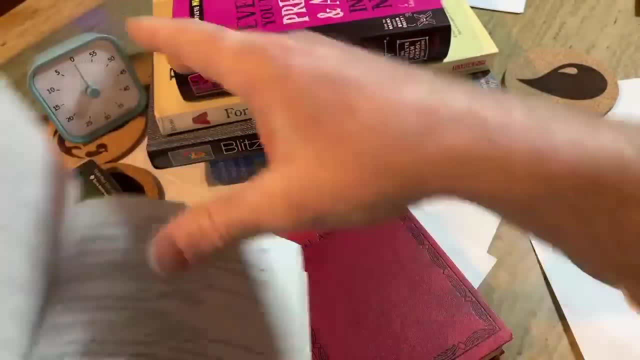 shipped from india. i'll leave a link in the description to a reprint. this is a reprint as well. this is not the original. it's higher algebra by bernard and child and i'm sorry, i just gotta smell it because it has an intoxicating smell. just ah, smells so good smells, so it's probably. 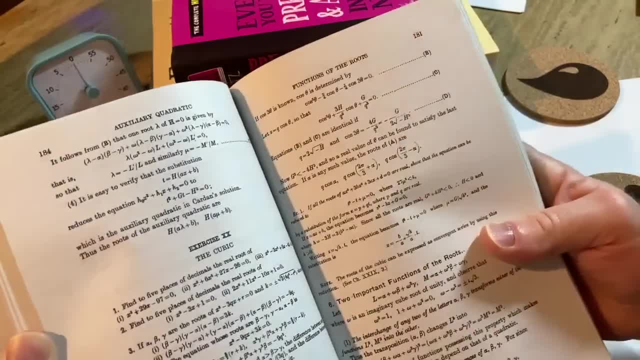 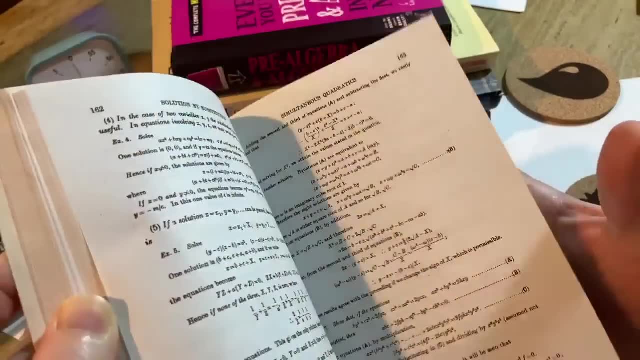 not good for me, but it smells really good and it's just got a lot of advanced mathematics that you're not going to see in college. you can get a math degree in a university in the united states and a lot of this mathematics you won't see. this is really old. 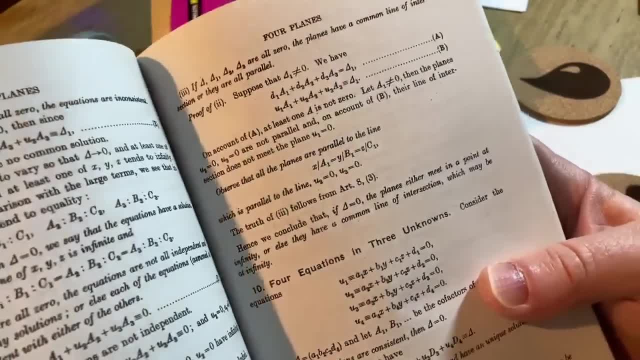 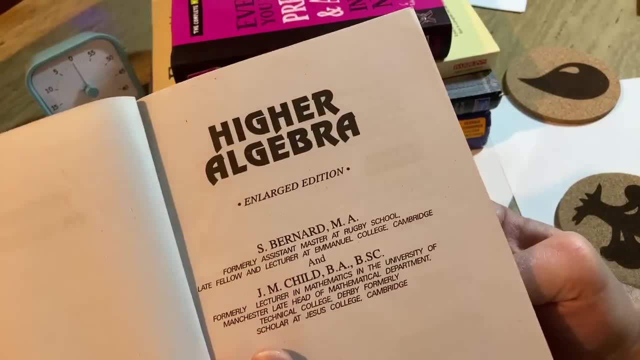 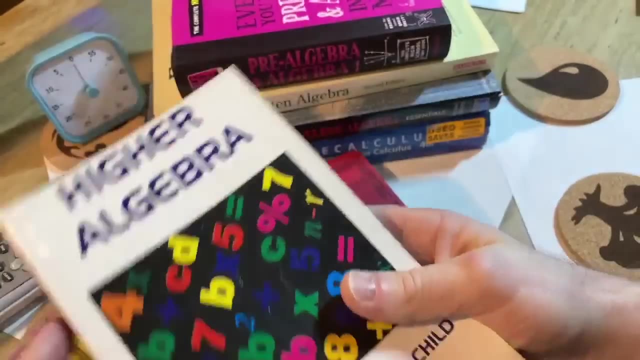 school. notice how small the lettering is, like the symbols. even though it's small, this is called the enlarged version, large edition. yeah, so it's got all kinds of weird stuff: continued fractions. it actually has calculus in it, so really interesting if you're looking for like tricky. 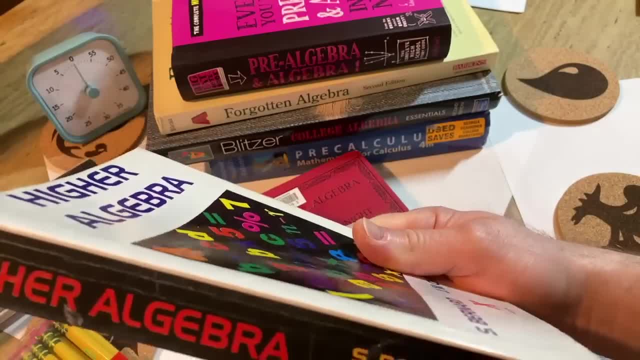 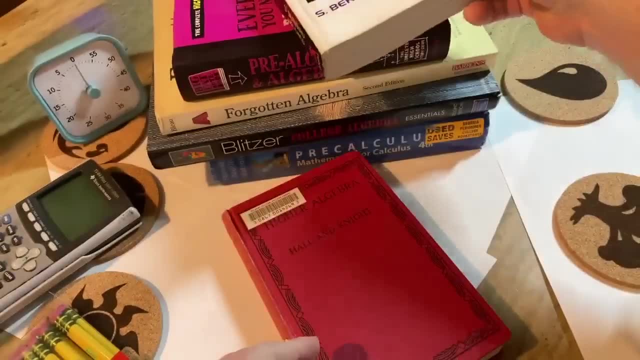 and challenging algebra problems. you could probably find problems in here and like: show them to your teacher and your teacher will help you out. but you know what i'm saying really well, your teacher won't be able to solve them because this book is ridiculous. um, then there is the. 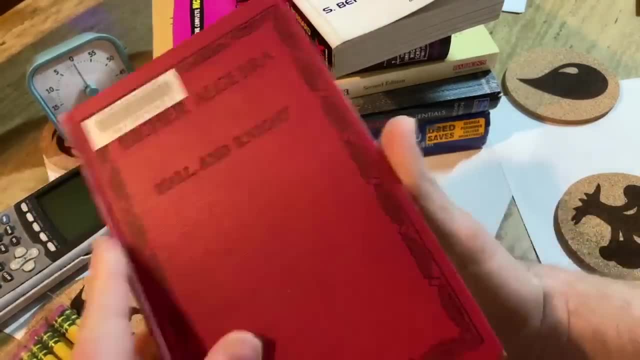 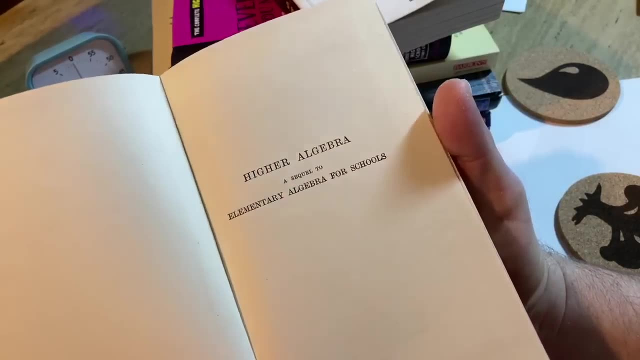 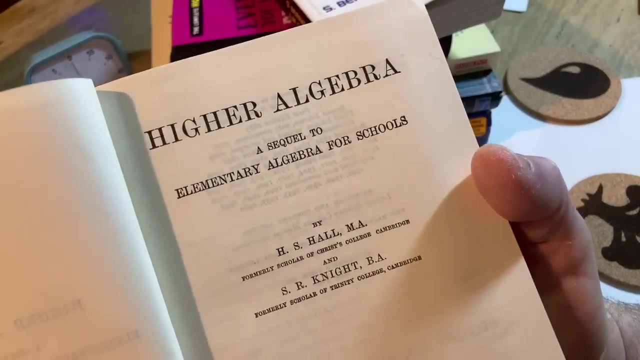 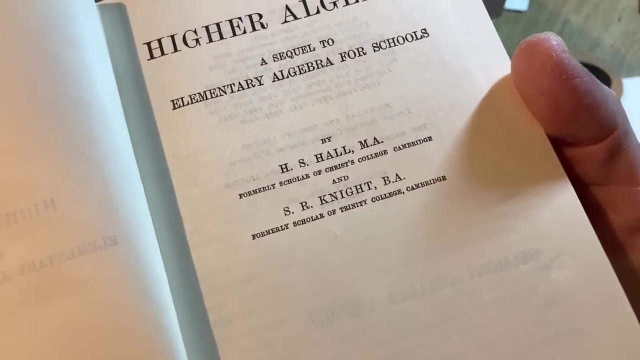 legendary higher algebra by hall and knight. this is an original copy. it's not a reprint but it's certainly not the first edition, a sequel to elementary algebra for schools. these are old british books. by the way, pretty sure i see cambridge hs hall, formerly scholar of christ's college, cambridge. wow, sr knight, formerly scholar of trinity college, cambridge. 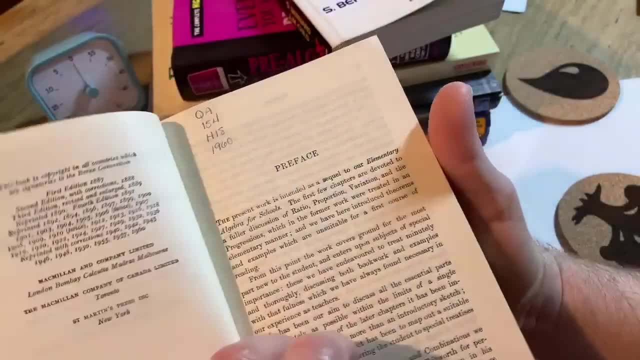 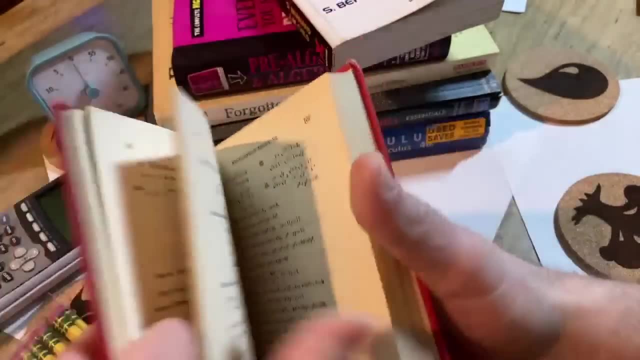 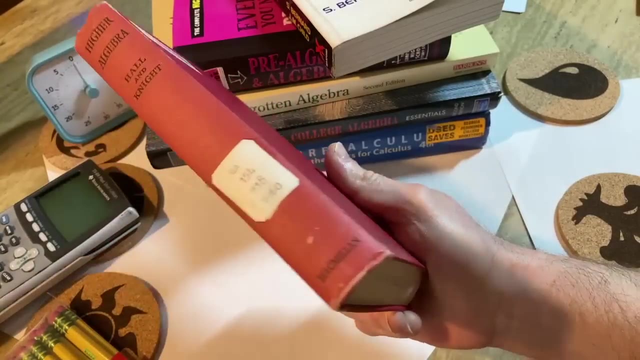 very, very fancy 1960 london, yeah, and very similar to um the bernard and child book, right. so very, very similar, similar style. plenty of extremely challenging exercises. uh, it's kind of like one of those fun books. i'll try to find this one. uh, if i find a reprint i'll leave it. it's harder to. 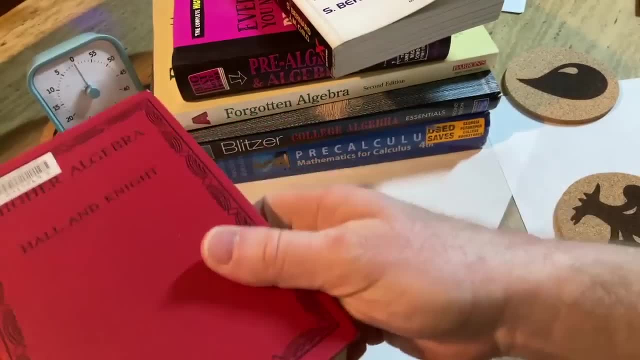 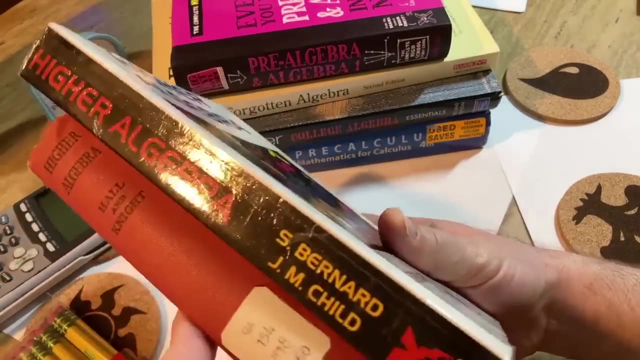 find affordable old copies, an old copy of the bernard and child. i haven't been able to actually find one, i've only been able to find reprints. so probably because they're books from you know- the uk, i believe- and so they're hard to get in in the 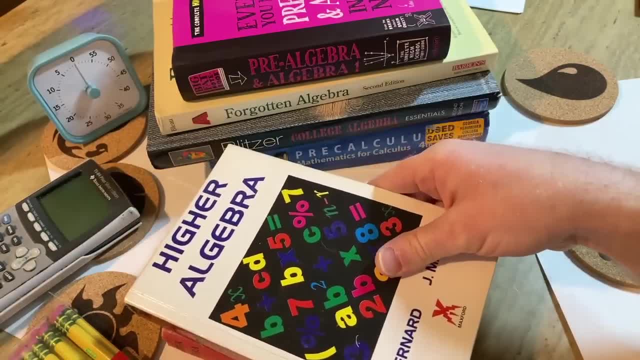 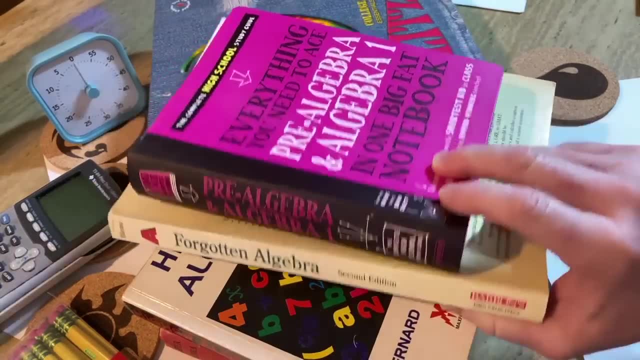 us. so those are some books that you can use to start from the beginning, again starting from the very beginning. you would, you would want to use one of these books here: pre-algebra and algebra one or, you know, forgotten algebra. these are great for beginners. and then the blitzer book, the 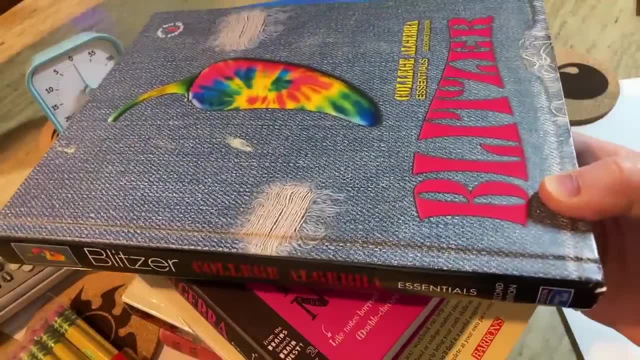 essentials version will save you money and it covers everything that's typically covered in a college algebra course in college. so if you're a beginner, you're going to want to use this book in college, and the pre-calc book covers everything that's covered. this is the one by stewart. 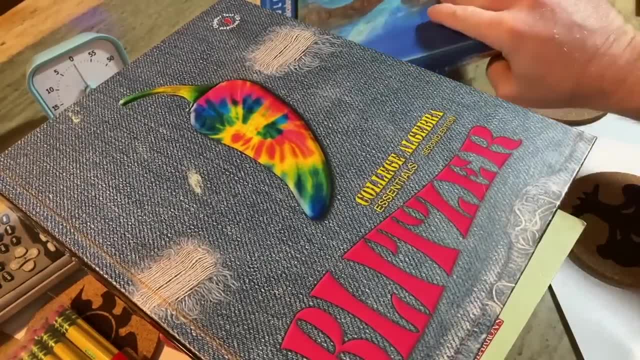 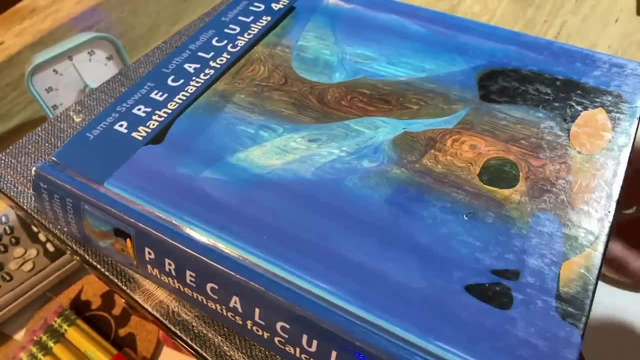 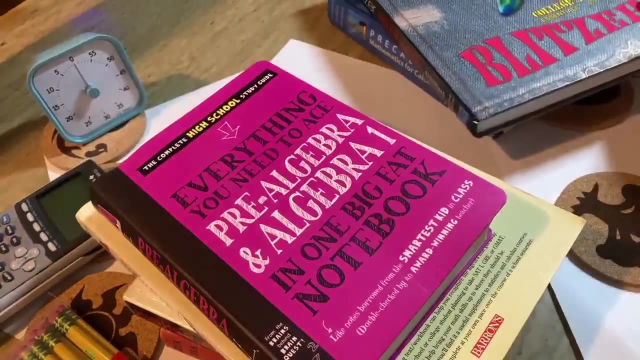 everything that's covered, uh, in a pre-calc course and a trigonometry course in college. so from the very beginning to the very advanced old school british style higher algebra books by bernard and child and hall and knight- those are classic books that contain um topics that you know. they 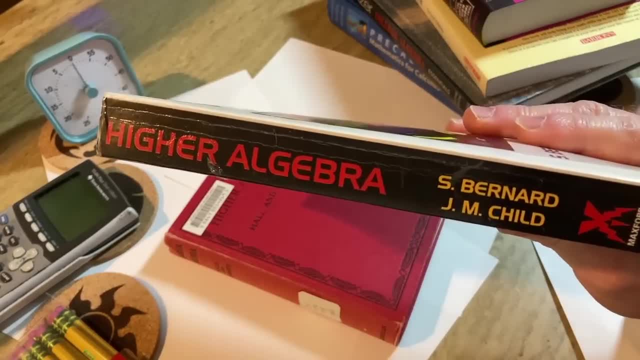 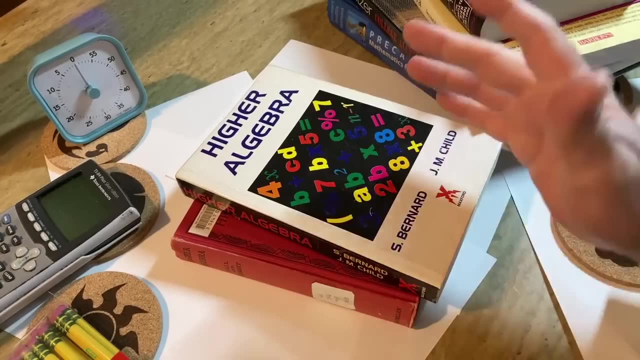 have continued fractions in there. ramanujan was famous for some of the things he discovered in continued fractions, and you can learn about them in these books on higher algebra. i also recommend the timer, so this is a timer that i use. i use this for multiple things. 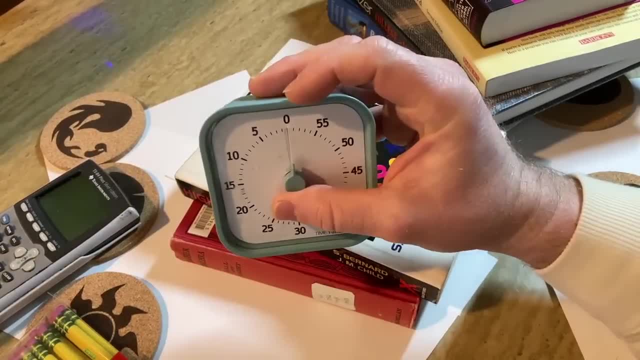 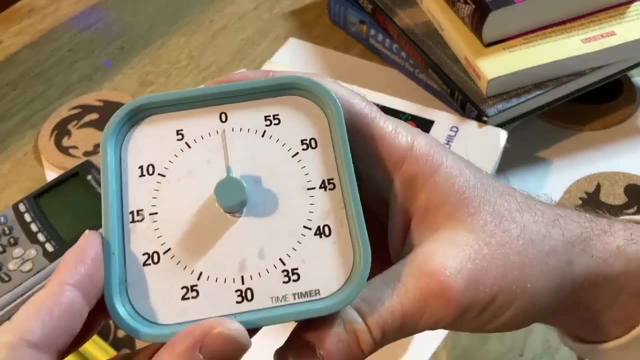 um, i used to use it for my laundry. i no longer use it for my laundry and i like it. it's simple. there's certainly more fancy timers. my phone has a timer, everyone's phone has a timer right, but this, you just set it and forget it right, and then when the time runs out. 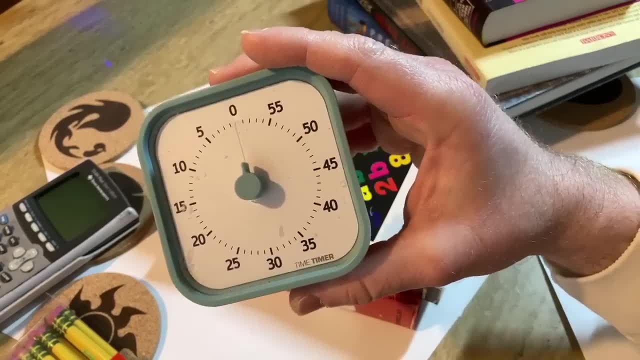 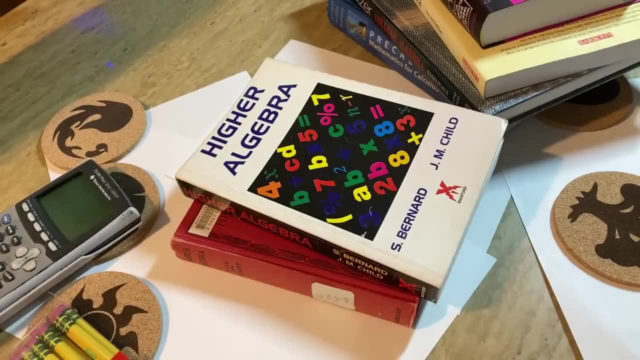 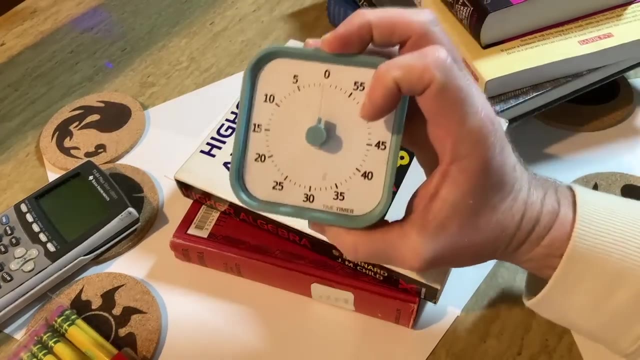 and i think, um, it's perfect, or it does beep. i don't know if you can hear it, but it does beep. my microphone has noise canceling so you might not be able to hear the beeping. let me just. maybe you can hear it now. not sure if you can hear it, but yeah, so great for self-study it uses. 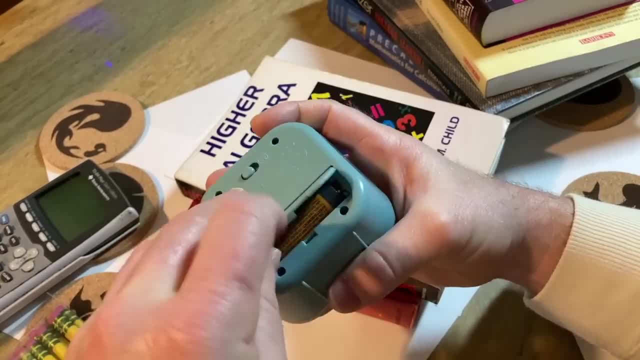 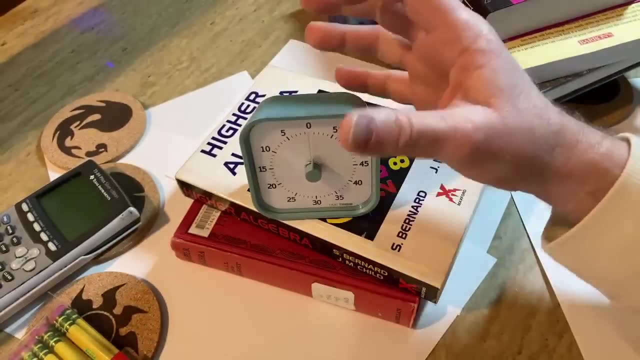 uh, one battery i believe, yeah, one double a battery. got an amazon basics battery in there and i use it for studying. i use it for uh for doing stuff, like if i want to make some videos for youtube or i want to work on some mathematics, just for. 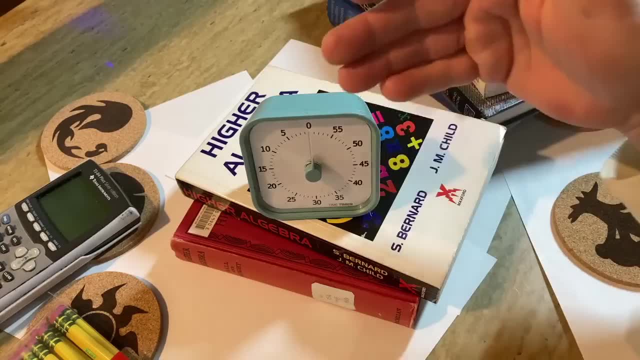 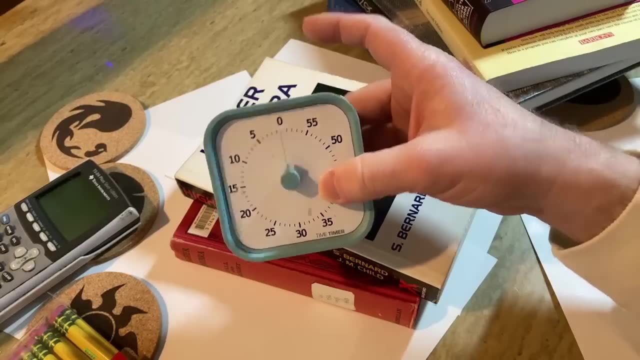 self-study. i like to do some math first thing in the morning, so i'll sit down for an hour 30 minutes and just work on some math, maybe read, and this makes sure that i don't overdo it and i don't underdo it. so it's just a nice way to time your sessions. it's not necessary, but it helps and i've 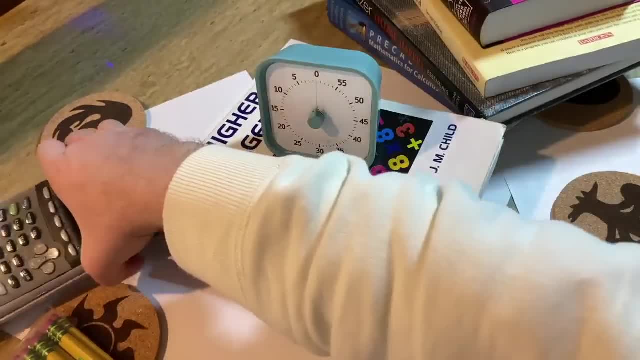 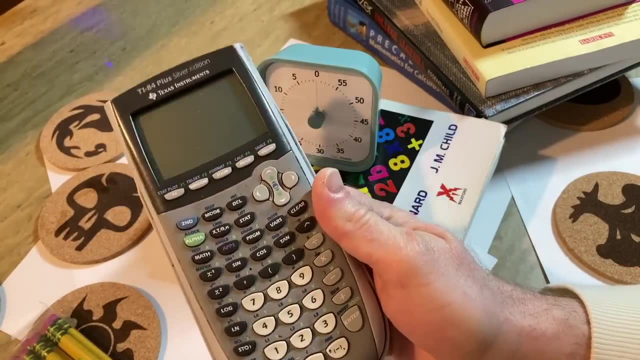 had it for a long time. i'll leave a link in the description. this is my calculator, the one i use. there are certainly newer ones and better ones. this one is really famous because, um, it doesn't have a computer algebra system. so if you're taking a class in college or high school, your teacher 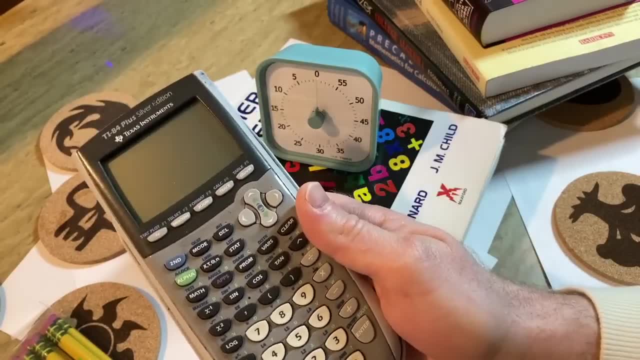 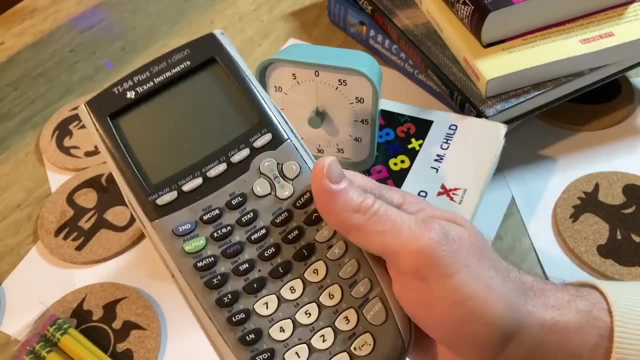 will probably let you use this one, whereas if you use a ti 89 or a ti inspire, those have computer algebra systems, so they actually do algebra for you, but teachers typically won't allow them. that's why this specific model, by the way, became so popular in the us. it's because teachers don't. 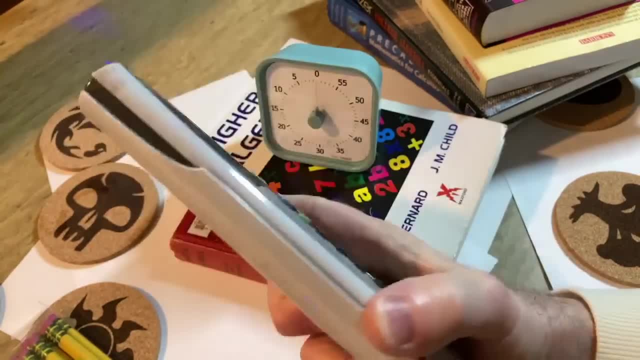 allow the other models. um, so it's kind of weird, right, kind of weird that, because teachers in general have a certain feeling: uh, a certain calculator you're going to be able to calculate how many times you're going to be able to calculate, how many times you're going to be able to calculate. 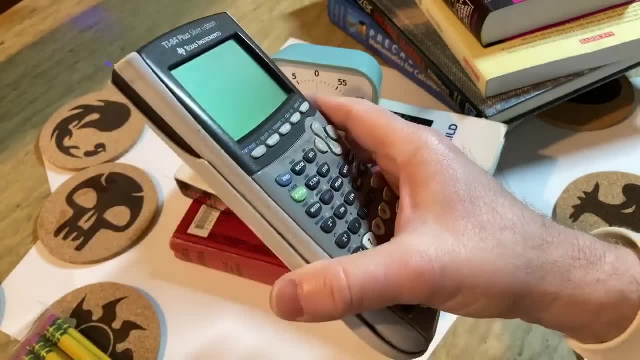 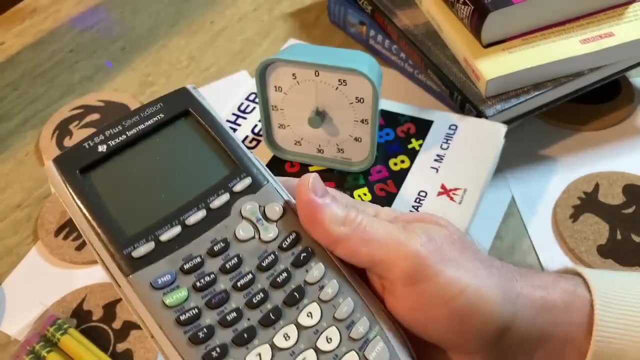 versus other calculators. kind of weird, kind of an interesting thing. personally, i don't care what calculator students use, it's just, you know, it doesn't really matter to me, but a lot of people do care. so something to keep in mind. um, very well made. i've had it for years. it's a beast. 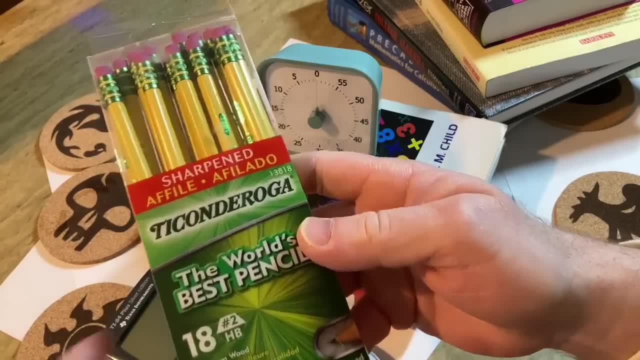 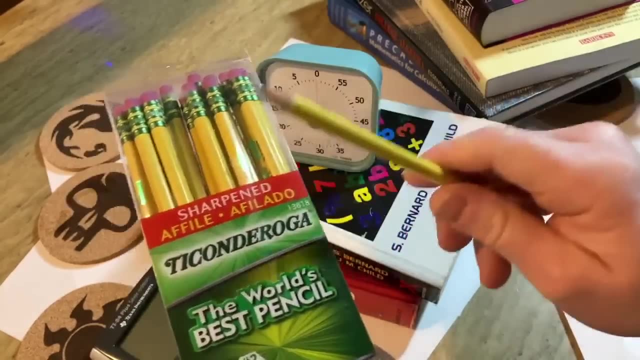 and then pencils. you need pencils to do math. these are my favorite pencils. i've been using these and, uh, this is almost a brand new pack. i've also been using these. these are just another brand paper mate. not as good as these. ticonderoga, the world's best pencil- awesome. 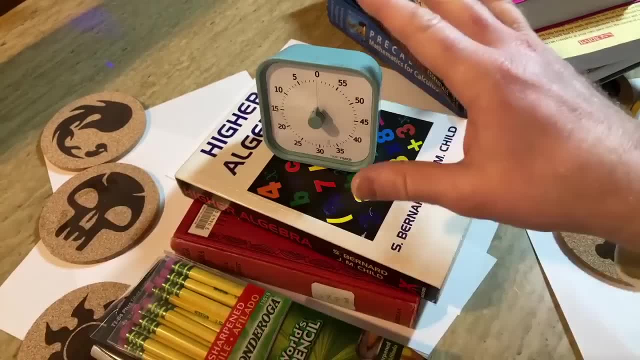 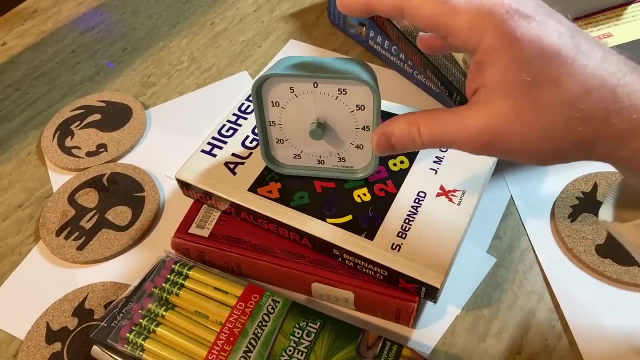 and then paper. i like to use paper with no lines. it kind of frees my mind. uh, the smartest guy i ever knew he. he didn't use lines on his paper and i remember studying with him and he was the first person i ever studied with. that ran circles around me and he had the 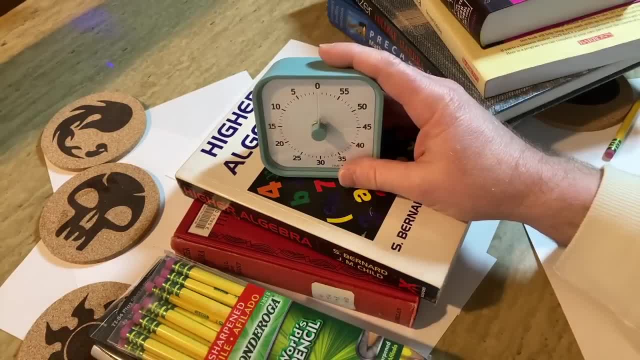 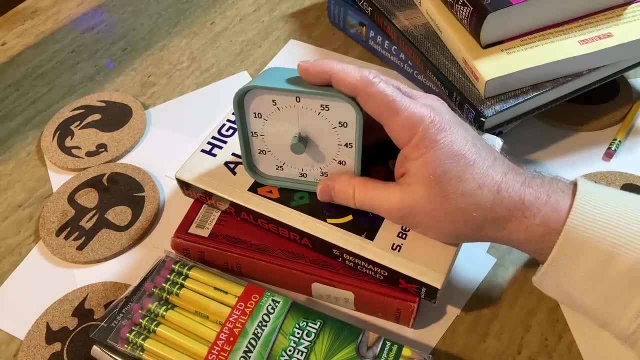 paper with no lines, i thought i'm gonna do what he does, you know, because, you know, learn from people who are better than you. so he was better than me, and so i decided to use paper with no lines. and here i am with paper with no lines, so i think it helps. and basic, non-electric, non-family. 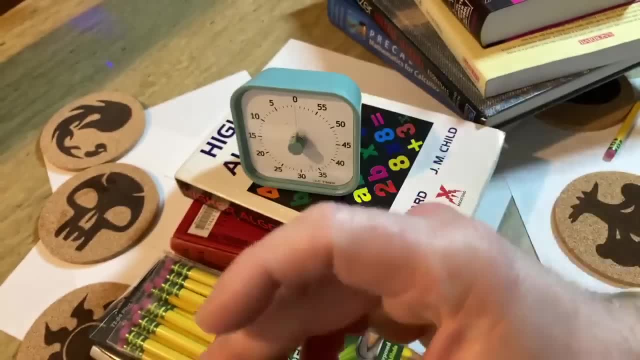 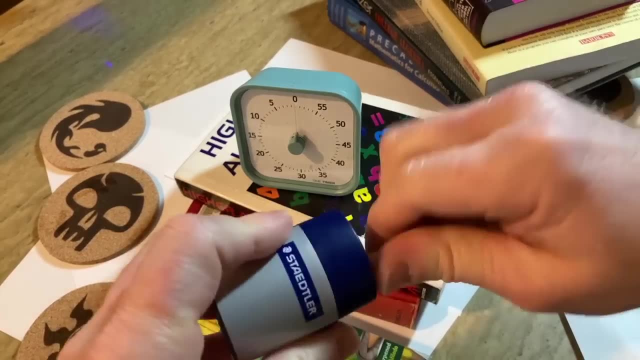 so you super affordable old school pencil sharpener. um, that way you don't have to plug it in. so if you're out in the woods and you're doing math or you lose power and you have some homework due and your teacher's not flexible, you can still light a candle and work on your physics. 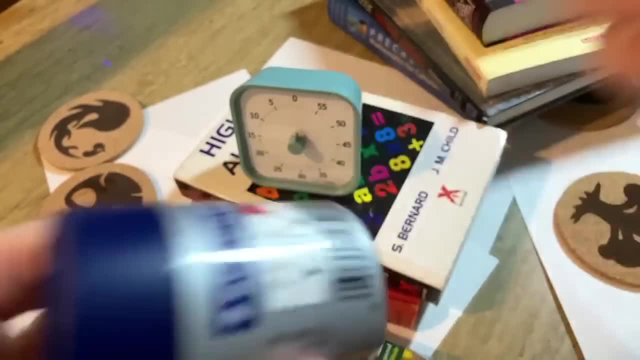 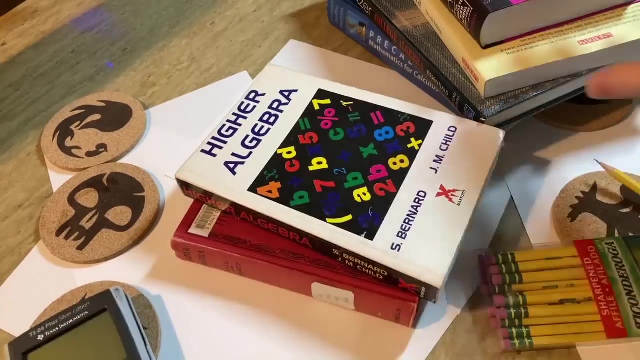 or math homework. i've actually done that, so that's a true story. anyways, rambling on forever about mathematics, i can talk forever about algebra. this video is about algebra and i hope this video has helped you. you can also take courses on algebra. there's all kinds of courses you can take.